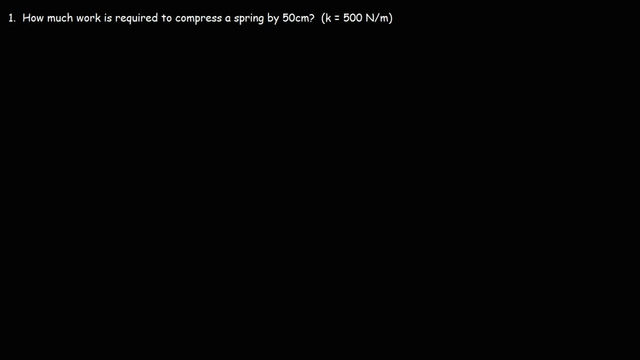 In this lesson we're going to talk about how to calculate how much work is required to compress the spring. So let's draw a picture. Let's say this is the original length of the spring And we want to apply a force in order to compress the spring. 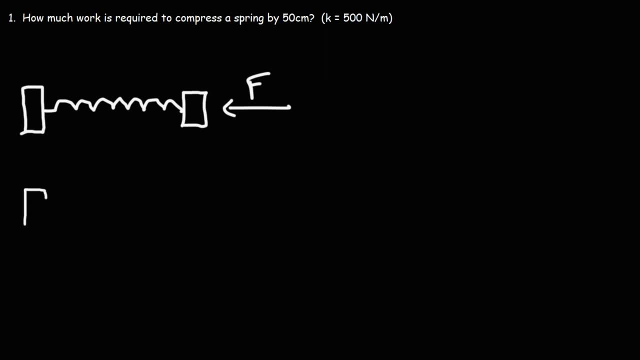 And we want to compress it by 50 centimeters, which is basically a half of a meter. So we want to compress it by 0.5 meters. How much work is required to do that? And we're given the spring constant K, which is 500 newtons per meter. 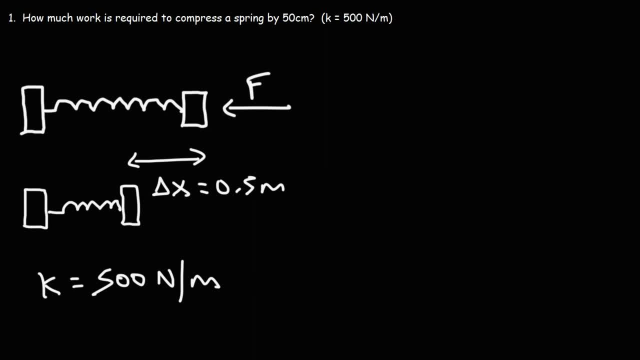 The spring constant tells you how stiff or how difficult it is to compress the spring. So what this value tells us is that, in order to compress the spring by one meter, we're going to require 500 newtons of force to compress it by just one meter. 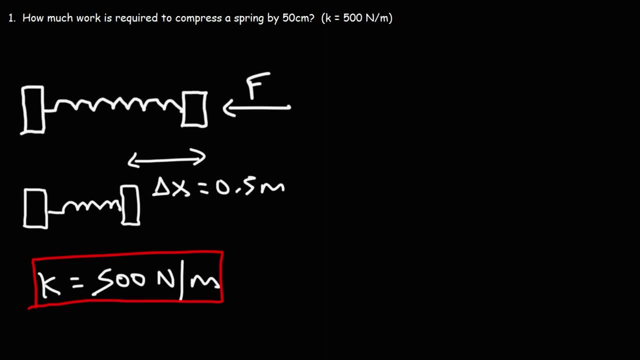 But how do we use this information to calculate the work done? The work done by a force is equal to the force times the force times the force. So, for instance, let's say if we have an object and we apply a force of 200 newtons, 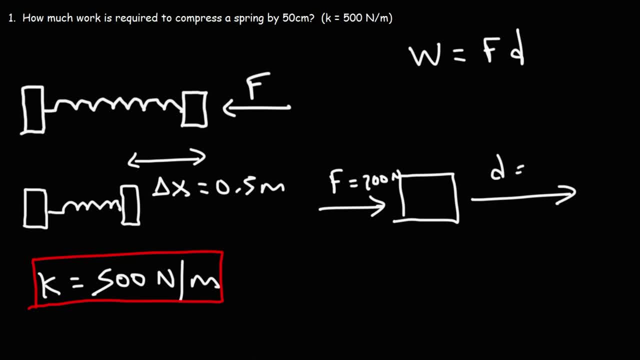 and we displace this object by five meters. the work done on that force, or the work done by that force, rather on this object, is 200 times five, which is a thousand joules. But this is the work done by a constant force. 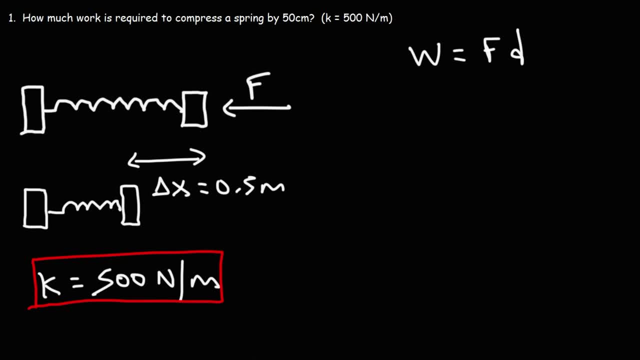 When we're compressing the spring, the force is equal to the force times the force. So the force that we need to do that is not constant. It's actually a variable force. That force increases As we apply a force to compress the spring, there is another force that is going against. 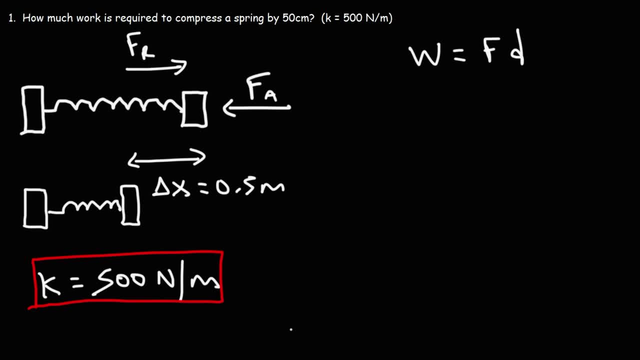 the force that we're applying, and this is called the restoring force. The restoring force is equal to negative KX. So the more you compress the spring, the magnitude of the restoring force increases, which means, to compress the spring, the force is equal to negative KX. 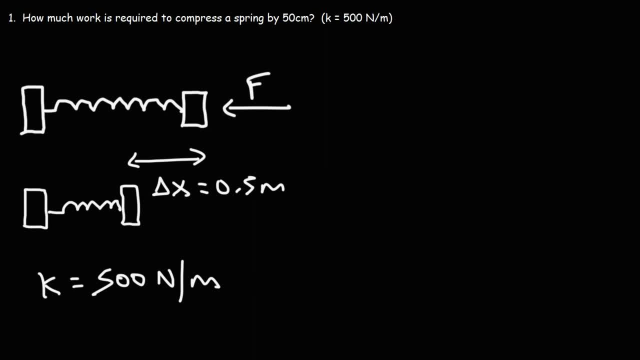 The spring constant tells you how stiff or how difficult it is to compress the spring. So what this value tells us is that, in order to compress the spring by one meter, we're going to require 500 newtons of force to compress it by just one meter. 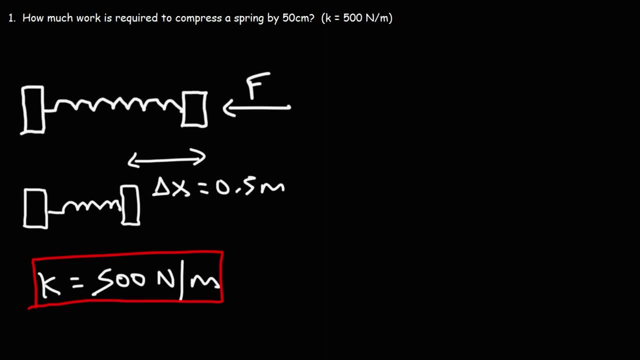 But how do we use this information to calculate the work done? The work done by a force is equal to the force times the force times the force. So, for instance, let's say if we have an object and we apply a force of 200 newtons, 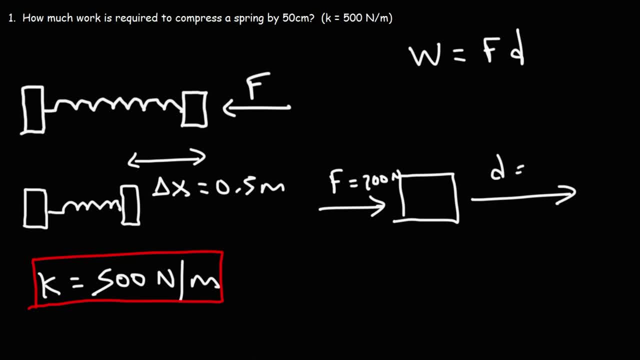 and we displace this object by five meters. the work done on that force, or the work done by that force, rather on this object, is 200 times five, which is a thousand joules. But this is the work done by a constant force. 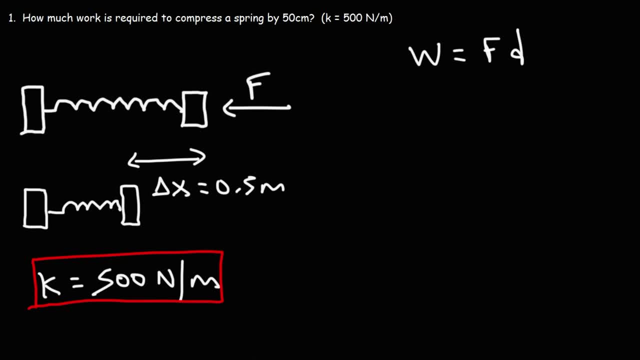 When we're compressing the spring, the force is equal to the force times the force. So the force that we need to do that is not constant. It's actually a variable force. That force increases As we apply a force to compress the spring, there is another force that is going against. 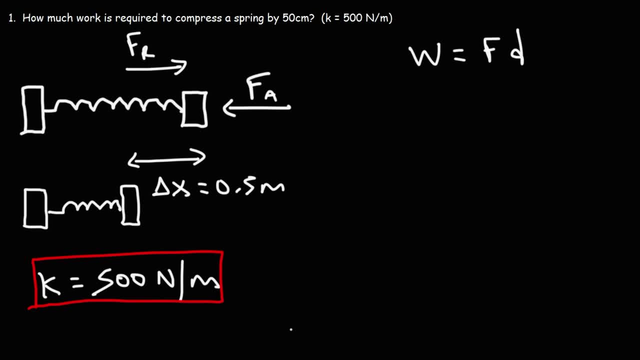 the force that we're applying, and this is called the restoring force. The restoring force is equal to negative KX. So the more you compress the spring, the magnitude of the restoring force increases, which means, to compress the spring, the force is equal to negative KX. 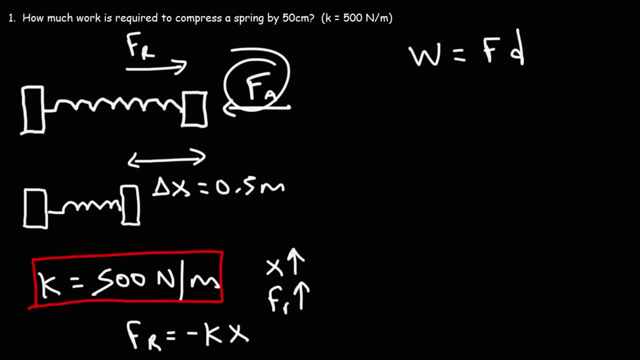 And for the spring further, you have to increase this applied force. So here's the relationship between the force applied and the distance at which you compress the spring. That force increases. That force is equal to KX. It's equal but opposite to the reactive force or the restoring force. 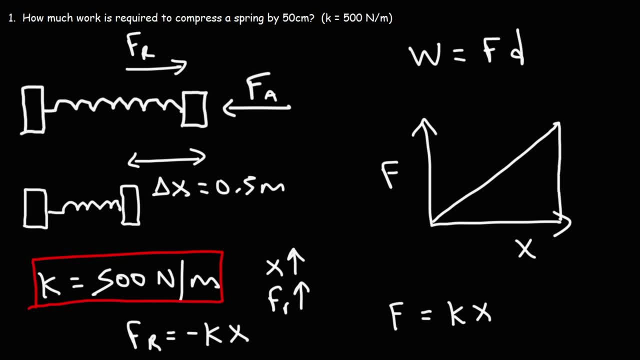 the work done by this variable force. what we need to do is calculate the area under the curve. The area for a rectangle is length times width, but for a triangle. 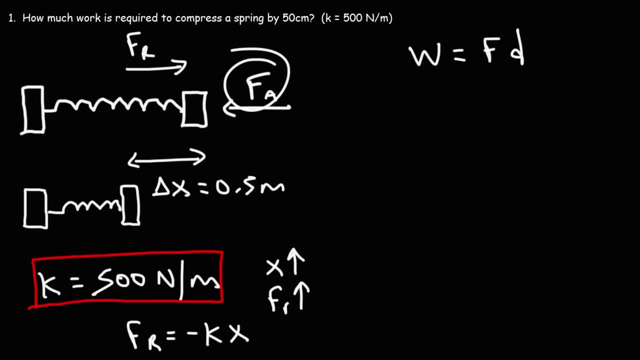 The restoring force is equal to negative KX. If you want to bring the spring further, you have to increase this applied force. So here's the relationship between the force applied and the distance at which you compress the spring. That force increases. That force is equal to KX. 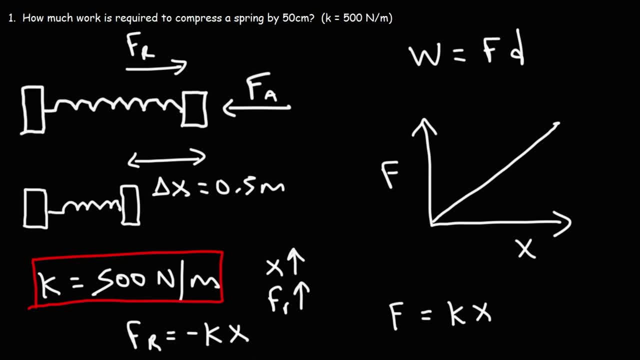 It's equal, but opposite to the reactive force or the restoring force. If we want to capture the force, we have to compress the spring at the same distance, And if we want to copy the force, we have to compress the spring, So that force is equal to negative KX. 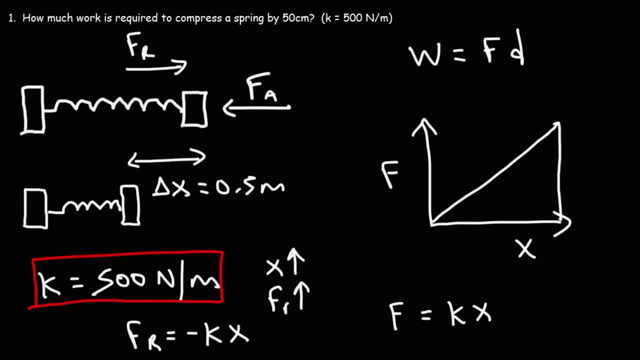 the work done by this variable force. what we need to do is calculate the area under the curve. The area for a rectangle is length times width, but for a triangle it's one half base times height. The base of the triangle is x, the height is the. 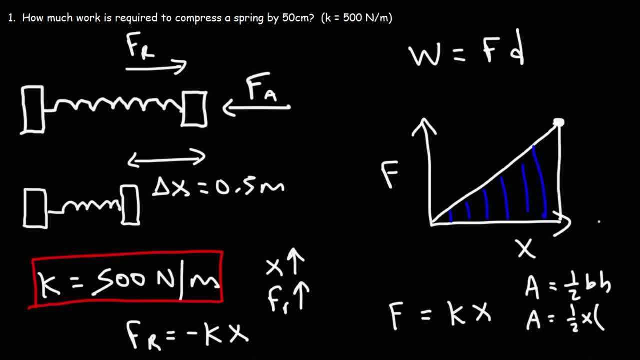 force. Let's say, if we focus on this point And we can replace the force with kx, So the area under the curve is one half x times kx, or in other words one half kx squared. Notice that this is the equation for the potential energy of a. 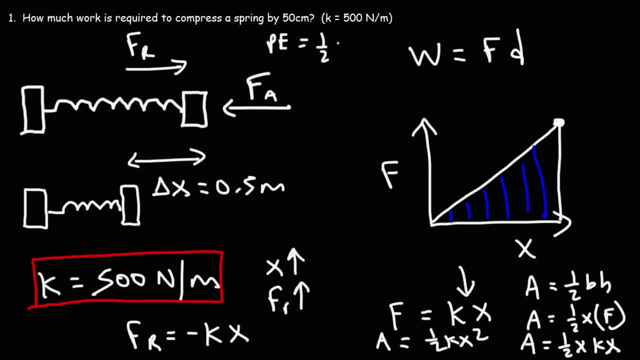 spring. If you want to calculate the elastic potential energy, it's equal to one half kx squared, which is equal to the work required to compress the spring. As you apply a force to compress the spring, that's what we're going to do. So we're going to apply a force to compress the spring. 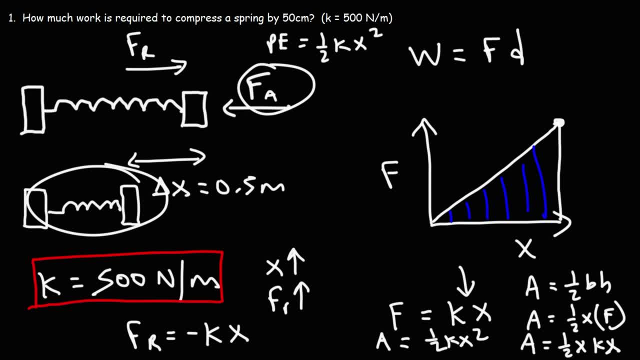 That's what we're going to do. So we're going to apply a force to compress the spring. That spring is acquiring potential energy And that energy comes from the force doing work on the spring. So the work required to compress the spring is equal to the potential. 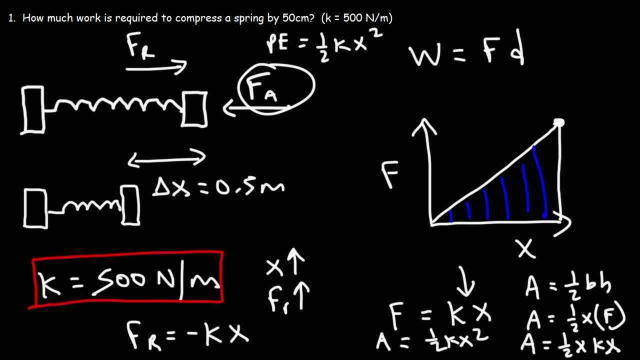 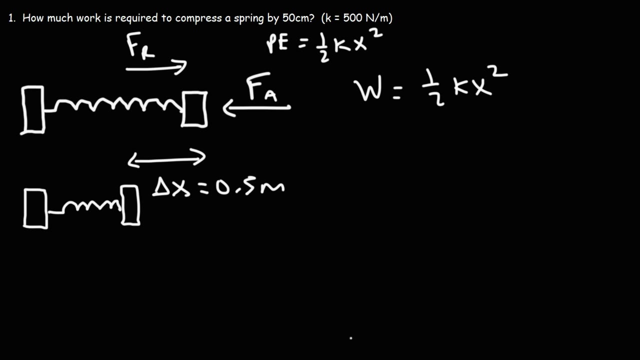 energy gained by compressing that spring. So we could use this formula to get the answer: The work required to compress the spring is one half kx squared. For those of you who want to use calculus to get the same answer or the same formula, here's what you can do. So, starting with this equation, 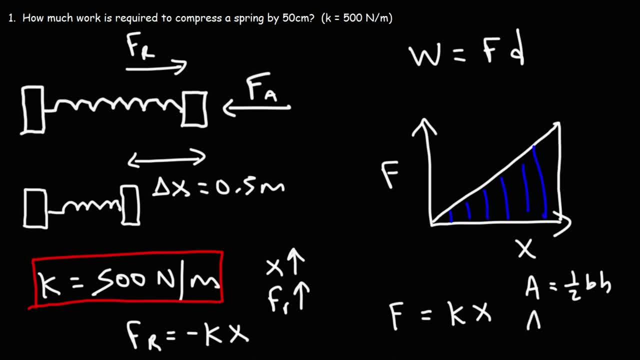 it's one half base times height. The base of the triangle is x, the height is the force. Let's say, if we focus on this point and we can replace the force with kx, So the area under the curve is one half x times kx, or in other words one. 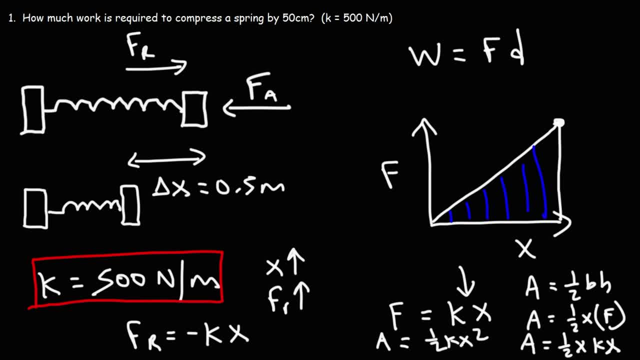 half kx squared. Notice that this is the equation for the potential energy of a spring. If you want to calculate the elastic potential energy, it's equal to one half kx squared, which is equal to the work required to compress the spring. 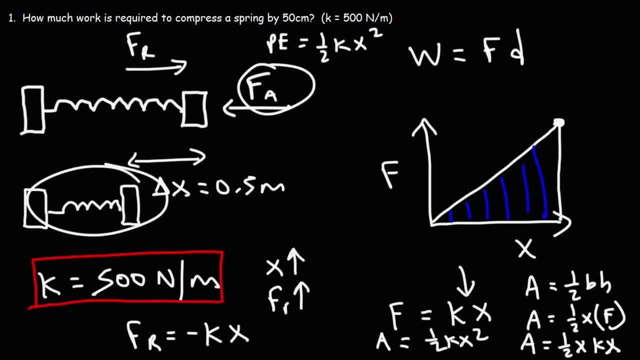 As you apply a force to compress the spring, that's spring is acquiring potential energy And that energy comes from the force doing work on the spring. So the work required to compress the spring is equal to the potential energy gained by compressing that spring. So we could use this formula to get the answer: The work required to 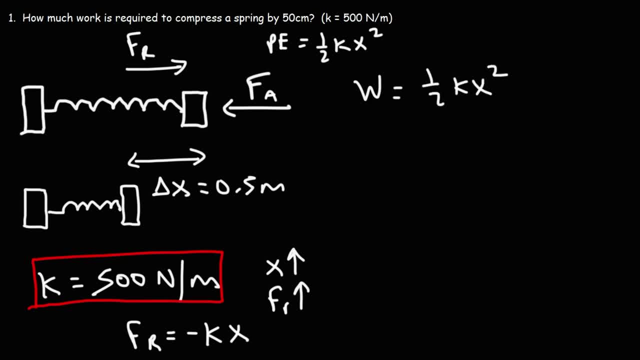 compress the spring is one-half kx squared. For those of you who want to use calculus to get the same answer or the same formula, here's what you can do. So, starting with this equation we have: dw is equal to f, dx, where the displacement is basically x, because we're 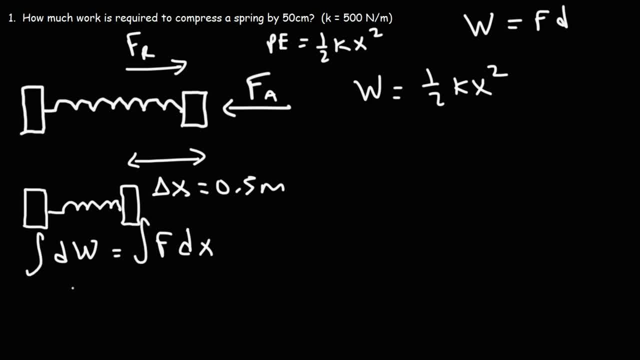 moving in the x direction. If we integrate both sides of this function on the left, we'll get the work which is the integral of the force function times dx. Now the force function we know it's f is equal to kx, So f is just kx. Now k is a constant. 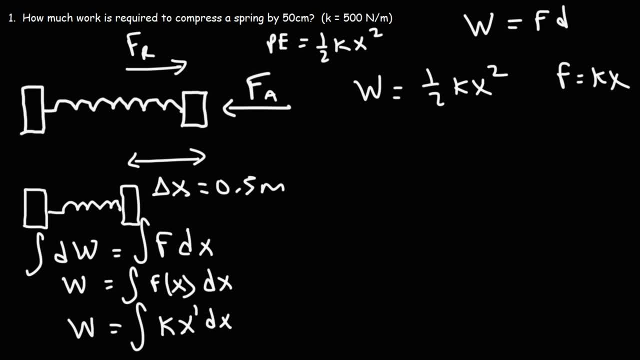 so we don't have to worry about that. So what we're really doing is we're integrating x to the first power Using the power rule. it becomes x to the second power. you add one and then divide, And then divide by this result And, of course, plus some constant c. 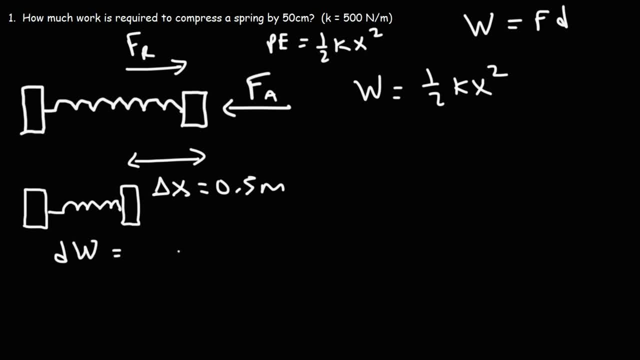 we have dw is equal to f dx, where the displacement is basically x because we're moving in the x direction. If we integrate both sides of this function on the left, we'll get the work Which is the integral of the force function times the x, Now the force function. we know it's. 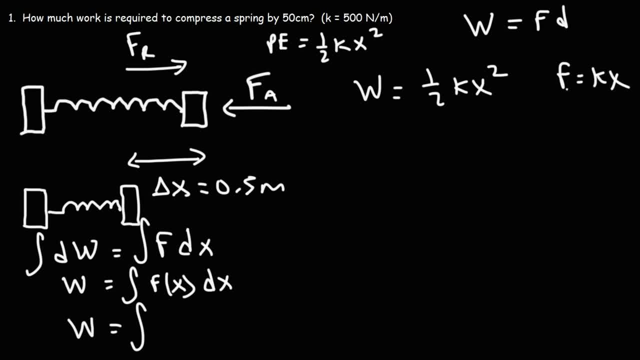 f is equal to kx, So f is just kx. Now, k is a constant, so we don't have to worry about that. So what we're really doing is we're integrating x to the first power, Using the power rule. 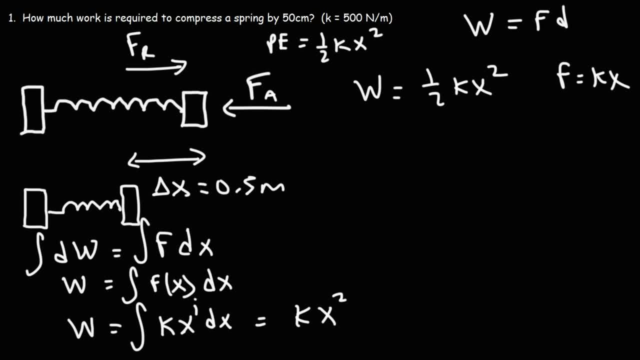 it becomes x. to the second power you add one and then divide by this result. Remember, we've done some Evergrande error here, but we have Input X squared, which is 1 half, as well as, again, the constant g squared. 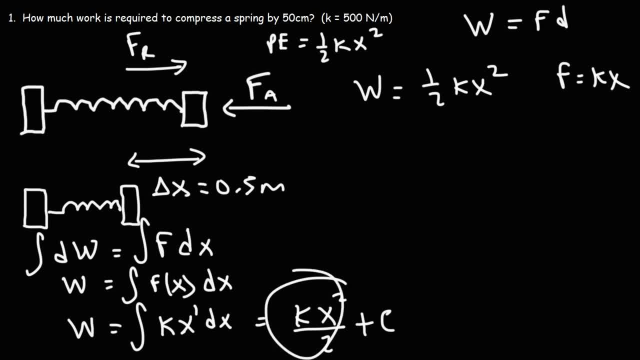 So this extended the Aunt Two case of the problem. So this time the equation will give us the Work Required, which is one half kx squared. So that's the other way in which you could get that formula. But now let's go ahead and finish this problem. 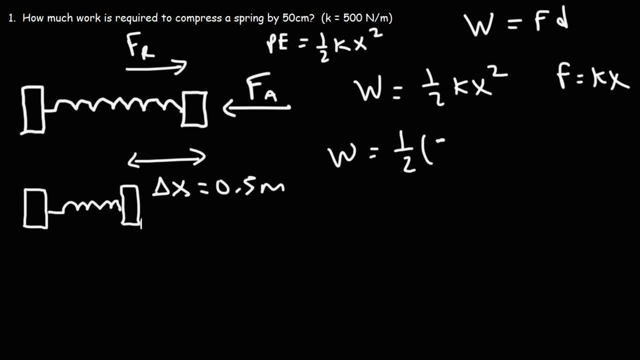 We have one half times k, k is 500.. Newtons per meter And then x squared, so X is 0.5 meters and we're going to square, so focusing on the units. K is Newtons per meter and then x squared, that's meters times meters, so you end up. 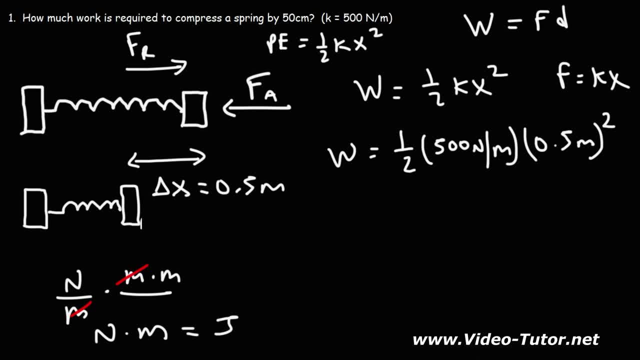 getting Newtons times meters, which is the jewel. so 1 Newton times 1 meter gives you one jewel. 0.5 times 500 times 0.50 squared, that's 62.5 joules. so that's how much work is required to compress the spring by 50 centimeters. so 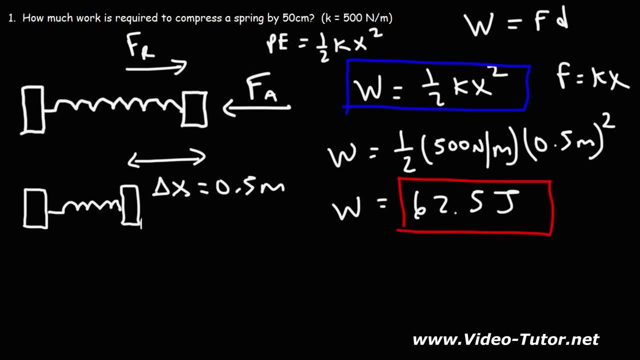 this is the formula that you need in order to calculate the answer.